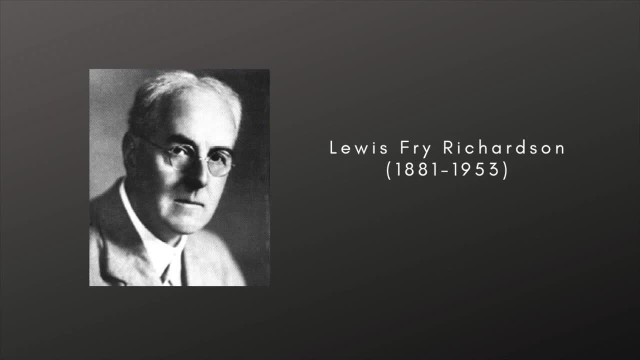 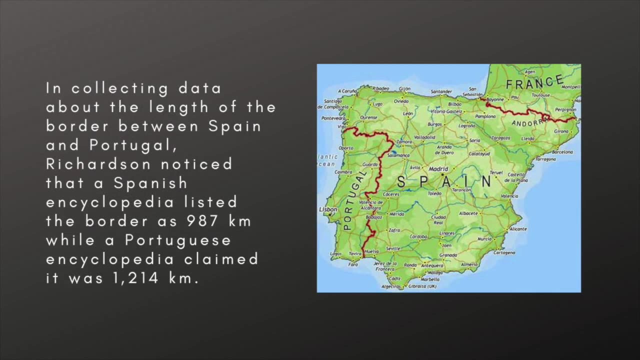 discrepancies between the values quoted by different sources. The length of the Spanish-Portuguese border, for instance, was once said by the Spanish authorities to be just 987 kilometers long, while the Portuguese gave it as 1,200.. Richardson realized that this kind of spread of measurements came about not because anyone was. 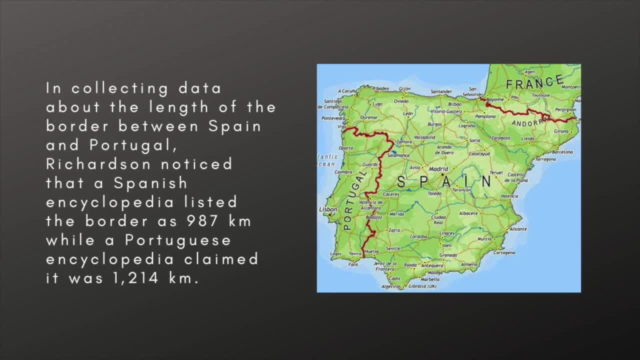 necessarily wrong, but because they were using different yardsticks or minimum length units in their calculations. Measure the distance between two points on a wiggly coastline or border with a ruler that's 100 kilometers long, and you'll get a smaller value than using a ruler that's half the. 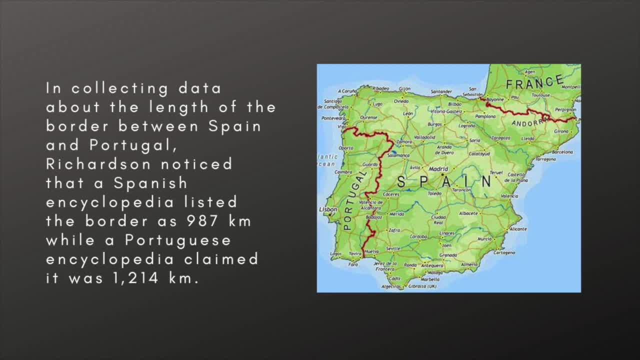 length. The shorter the ruler, the smaller the wiggles it can take into account and include in the final answer. Richardson showed that the measured length of a coast or border increased without limit as the yardstick or unit of measurement shrank, and shrank Evidently in the case of the Spain-Portugal. 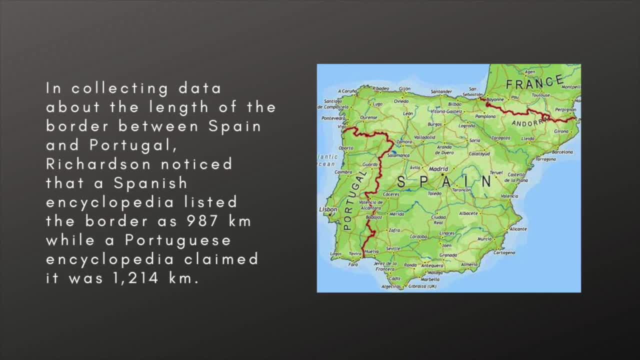 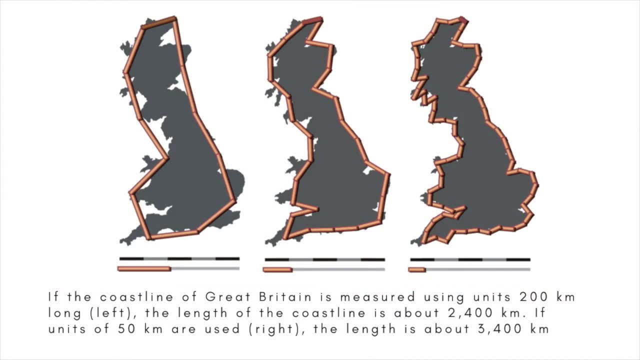 border, the Portuguese had done their measuring with a shorter length unit. At the time he published the paper he had written that the Spanish border was a short length unit. In 1961, no one paid much attention to this surprising discovery- what's now called the. 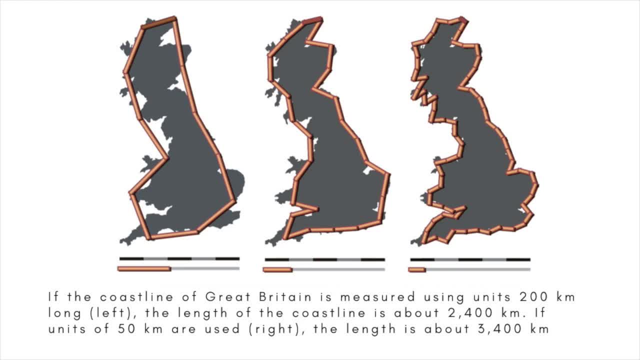 Richardson effect or coastline paradox. But looking back, it's seen as an important contribution to the development of an extraordinary new branch of mathematics which Mandelbrot, the man who made it famous, eventually described as beautiful, damn hard, increasingly unuseful. 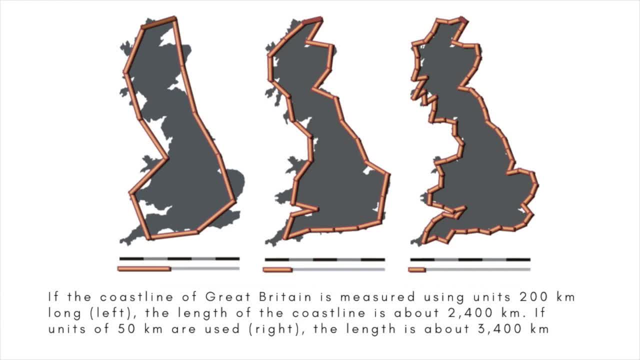 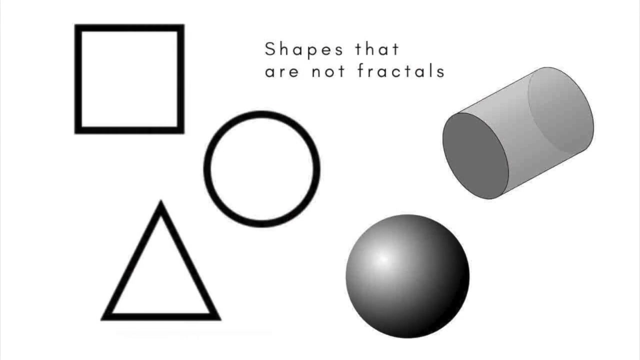 In 1975, Mandelbrot also coined a name for the weird things at the heart of this new field of research: fractals. A fractal is something such as a curve or a space with a fractional dimension. To be a fractal, all a shape needs is to have a complex structure at all scales, no matter how small. 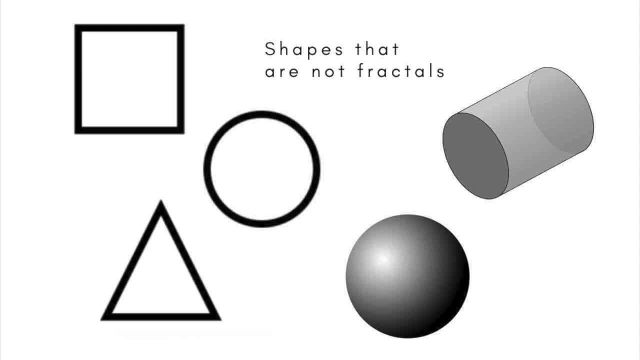 The vast majority of curves or geometrical figures we come across in maths aren't fractals. A circle, for instance, isn't a fractal because if we progressively zoom in on part of the circle's circumference, it looks more and more like a straight line. 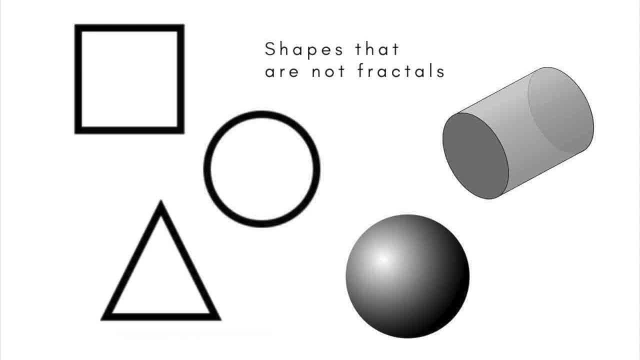 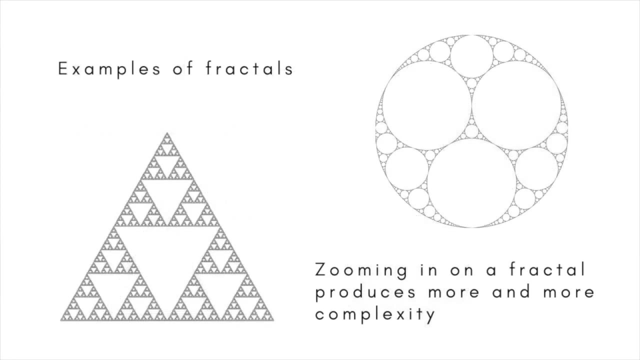 A square isn't a fractal either. for the same reason. It always retains its structure at the four corners, but everywhere else it looks just like a straight line after zooming in. To qualify as a fractal it isn't enough to have complex structure at one or finitely. 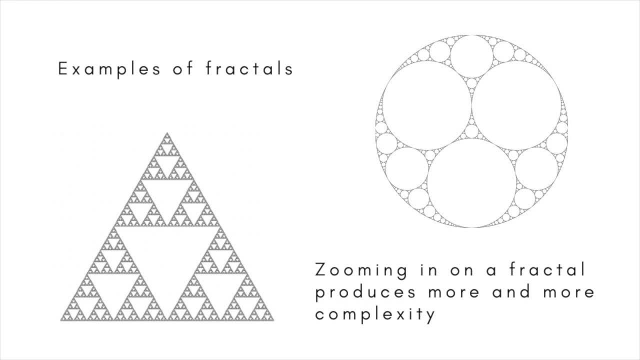 many points. There has to be that kind of structure at all points. The same is true of shapes in three or more dimensions. Spheres and cubes, for instance, aren't fractals, but there are many shapes in many different dimensions that are. 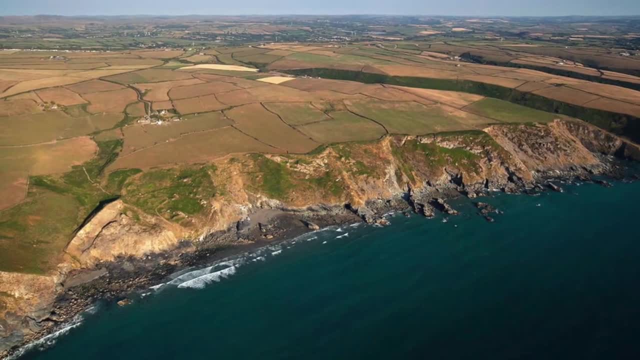 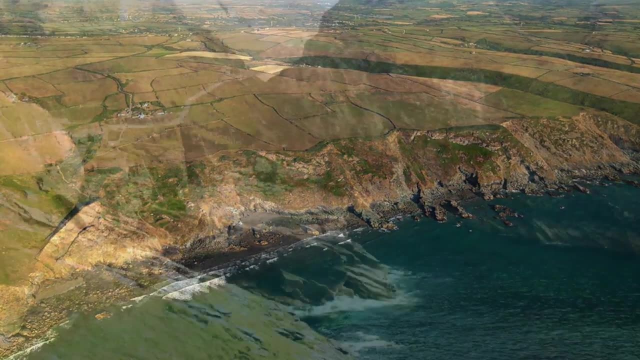 Going back to the coast of Great Britain, a small-scale map shows only the largest fractal in the world, The largest bays, inlets and peninsulas. Go to a beach, however, and you'll see much smaller features: coves, headlands and so. 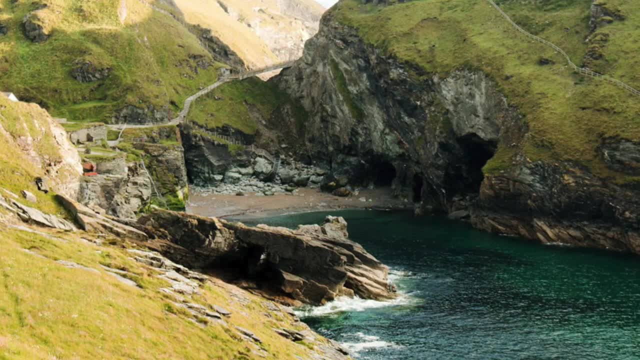 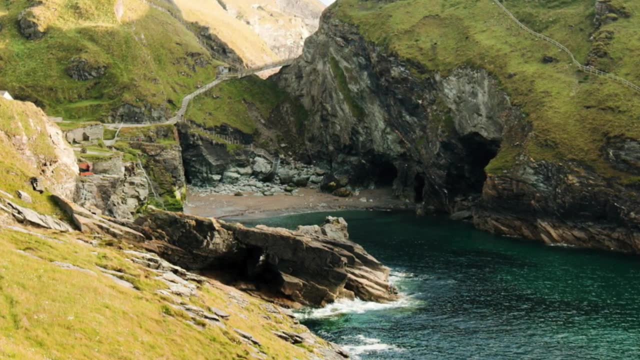 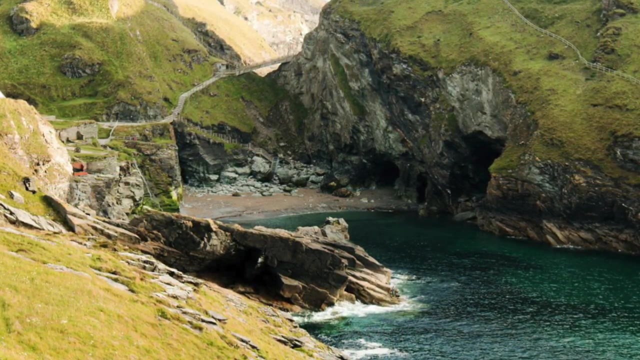 forth. Look even closer with a magnifying glass or microscope and you'd be able to discern the minuscule structure of the edges of every rock on the shore, down to smaller and smaller scales. In the real world, there's a limit to how far it's possible to zoom in. 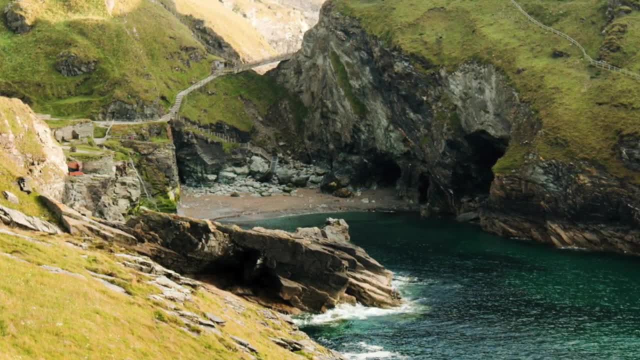 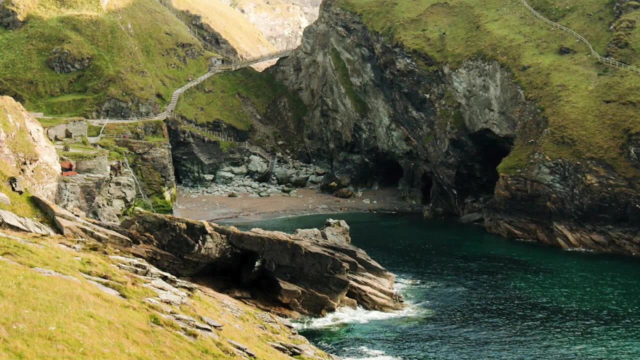 Below the level of atoms and molecules, and perhaps even worse. there's a limit to how far it's possible to zoom in. Well before then, it becomes meaningless to talk about more detail to do with the length of coastlines, and in any case the length changes minute by minute due to erosion and 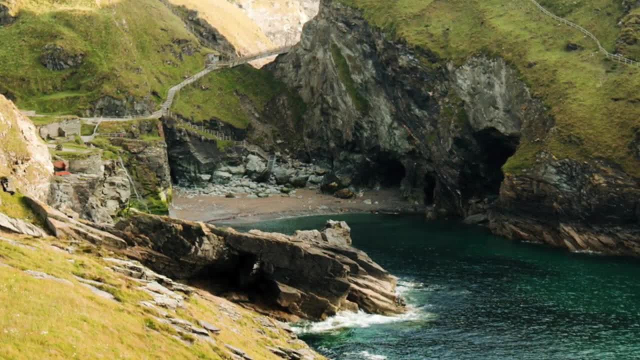 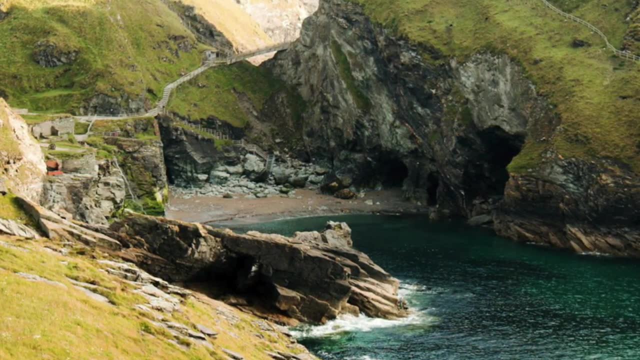 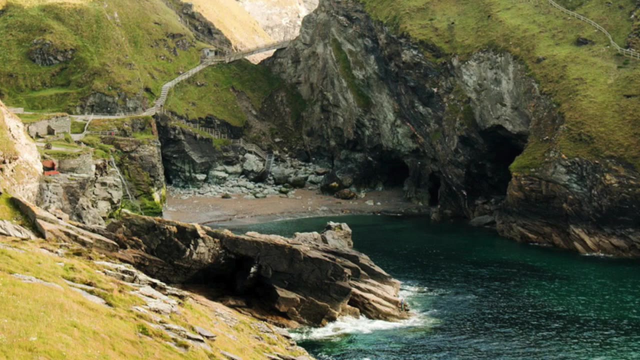 the ebb and flow of the tides. Nevertheless, the coast of Great Britain and the outline of other islands and countries are pretty good approximations to fractals, and this explains why different sources of data give different values for the length of borders. 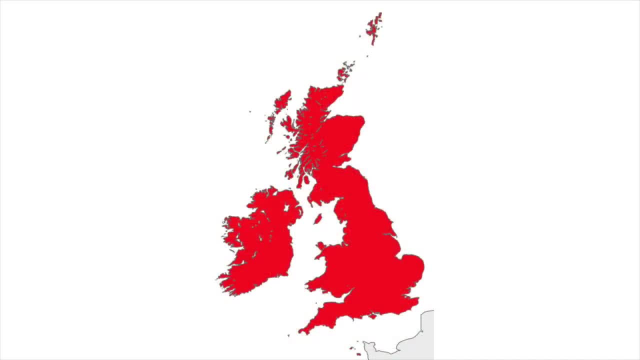 of borders. Looking at a map of the whole of Great Britain, you wouldn't be aware of all the little indentations that you'd see if you actually walked around the coast and so, based on the map, would come up with a much shorter length Simply strolling along the beach. you'd miss all the fine. structures of the rocks and get a much shorter length than if you used a foot-long ruler or something even more precise to measure all the little ins and outs at a small scale. The length actually grows exponentially rather than approaching ever more closely a final true. 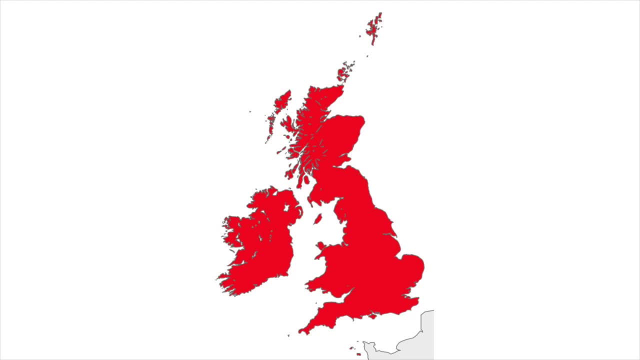 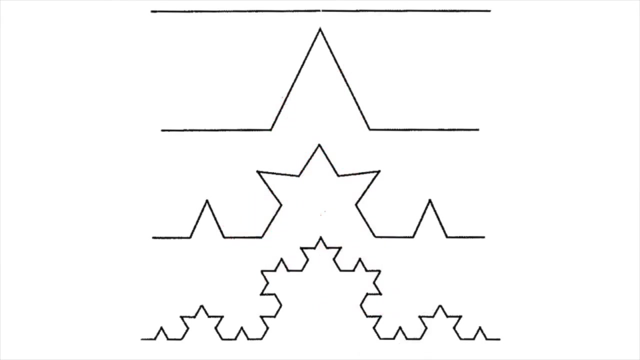 figure. In other words, if you use measuring equipment with enough resolution, the length you obtain can be as great as you like, again within the limits set by the atomic nature of matter. As well as natural fractal systems such as coastlines, there are many purely mathematical fractals. A simple way to make one. 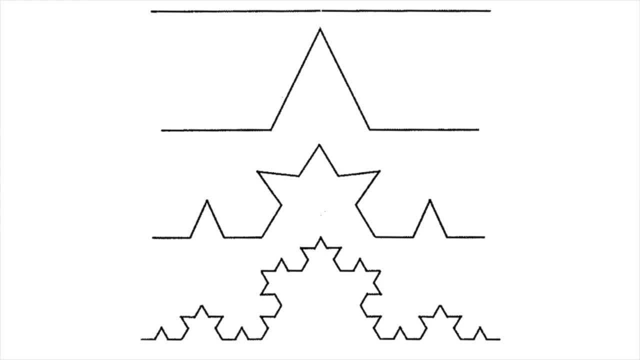 is to divide a line into three equal sections, draw an equilateral triangle pointing outwards that has the middle section as its base, and then remove the section that is the base. This process is then repeated, starting from each of the four resulting line sections. 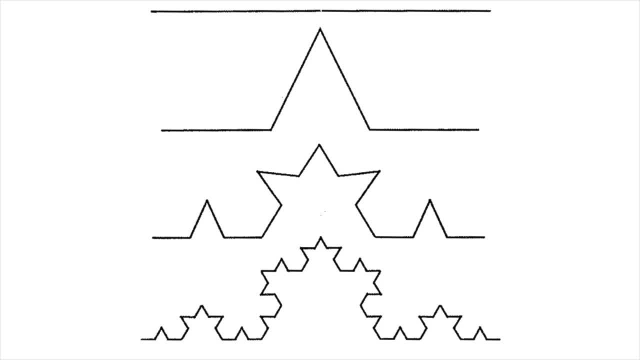 and repeated again for each of the new, shorter sections, and so on for as long as you like. The final result is known as the Koch curve, after the Swedish mathematician Helge von Koch, who wrote about it in a paper in 1904.. Three of these Koch curves can be joined to form what's. 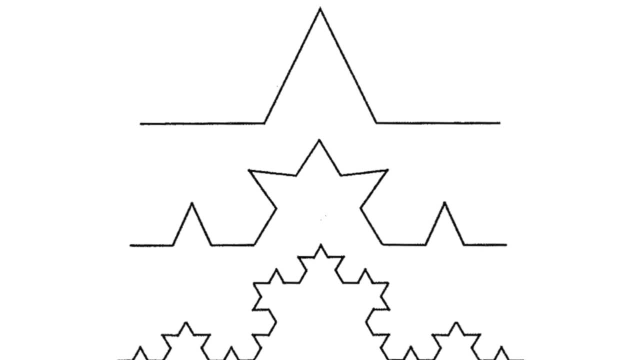 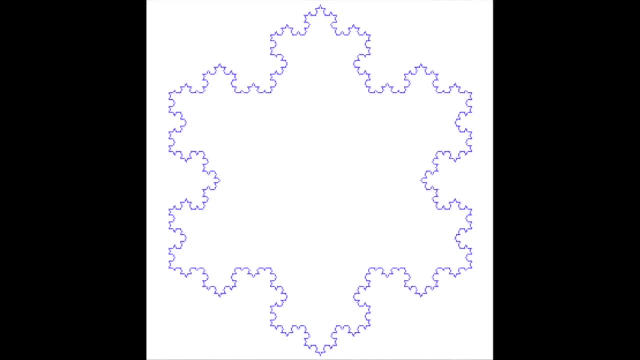 known as the Koch snowflake. The Koch curve was one of the earliest fractal shapes to be constructed. A couple of other now-familiar fractals were described mathematically in the first quarter of the 20th century. The first quarter of the 20th century was called the Koch. 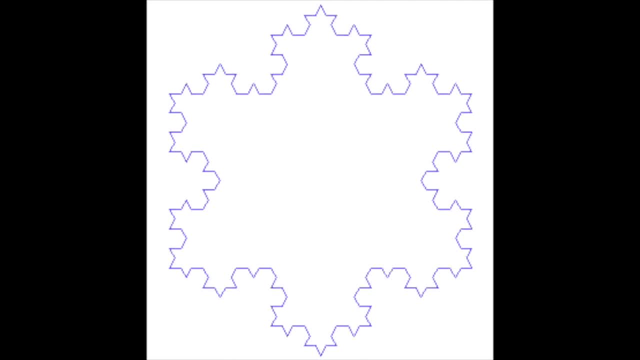 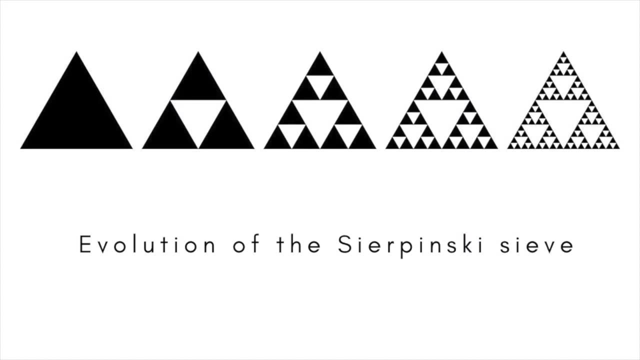 curve and the second quarter of the 20th century was called the Koch snowflake. The Koch curve was the first quarter of the 20th century by the Polish mathematician Vaclav Sierpinski, The Sierpinski sieve, or gasket and carpet To make the sieve. 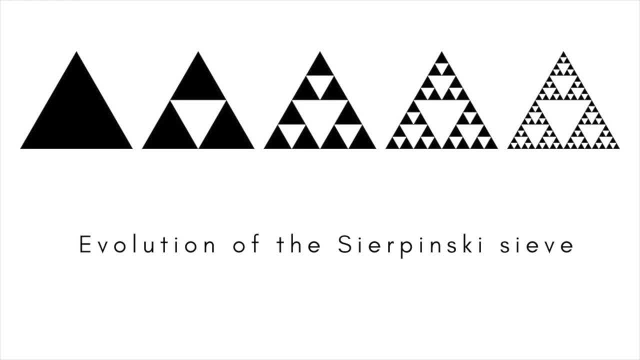 Sierpinski started with an equilateral triangle and divided it into four, each half the size of the original. Then he removed the central one to leave three equilateral triangles, repeated the process with each new triangle and kept on doing this over and over again. Although such objects 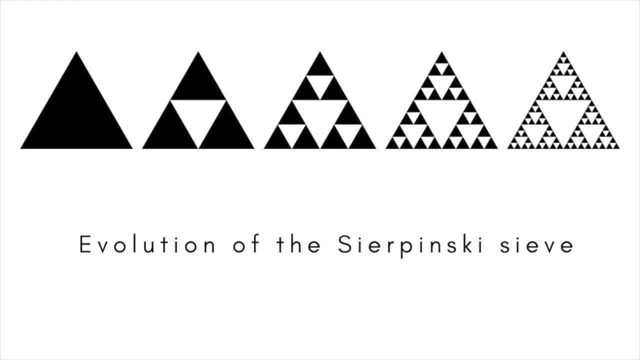 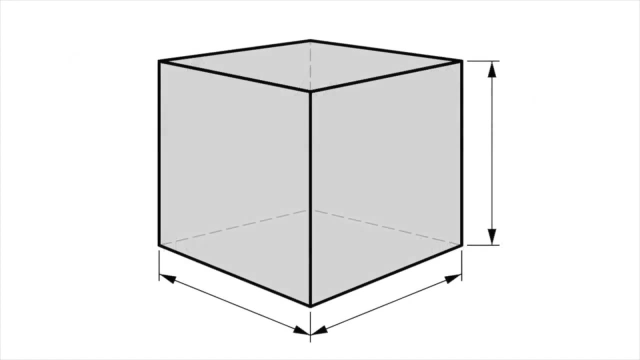 have been used for the first time. they have not been used for the second time. The first half of the Sierpinski sieve, for instance, appeared in Italian art going back to the 13th century. Among the most interesting and counterintuitive properties of fractals is their dimension On. 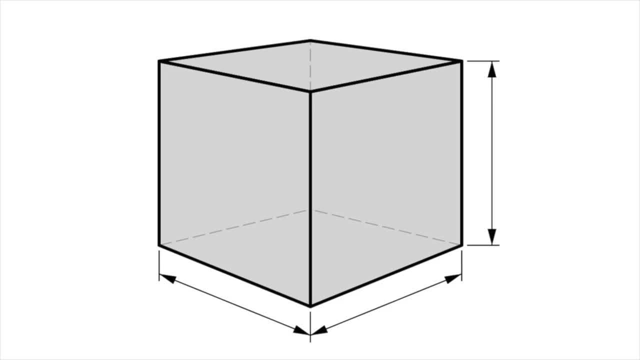 hearing the word dimension, a couple of ideas generally spring to mind, one to do with the overall size of something, as in the size of a fractal. The first half of the Sierpinski sieve, for instance, refers to the dimensions of a room and the other that refers to a unique spatial. 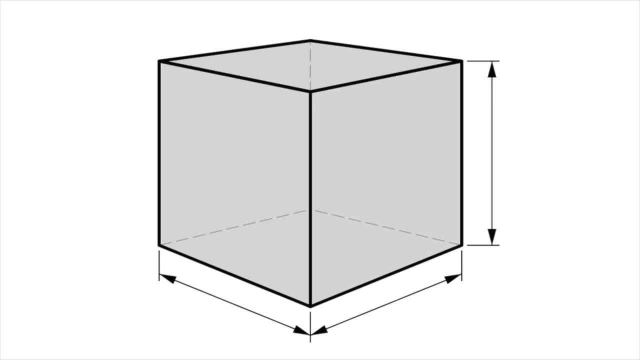 direction. We say that a cube is three-dimensional because it has sides that lie in three different directions at right angles to one another. This second intuitive understanding of dimension, which relates to the number of perpendicular directions it's possible to travel in, is roughly equivalent to what, in mathematics, is called the topological dimension A sphere has. 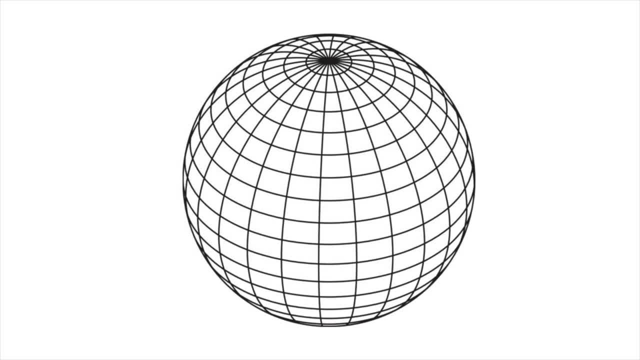 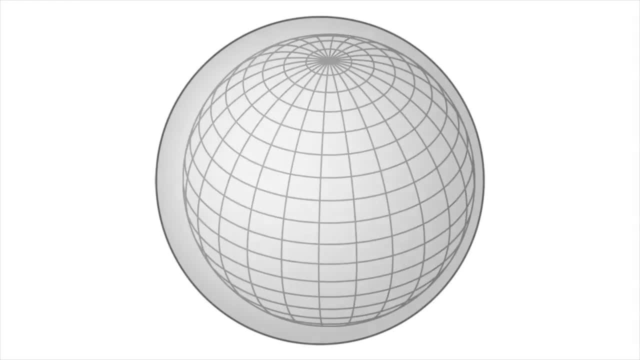 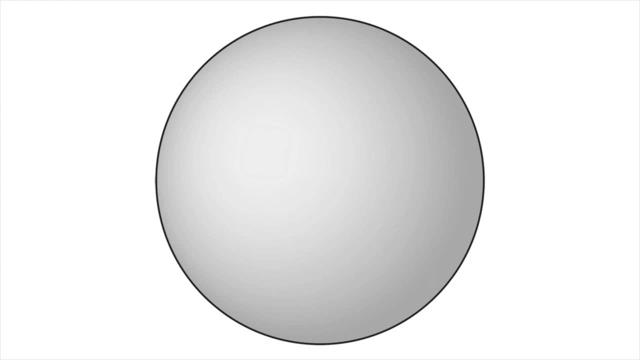 topological dimension two because we can travel along it in the directions given by north and south, or by east and west. A ball, on the other hand, has topological dimension three because it also has an up and down, where down is towards the centre and up is away from the centre, as on. 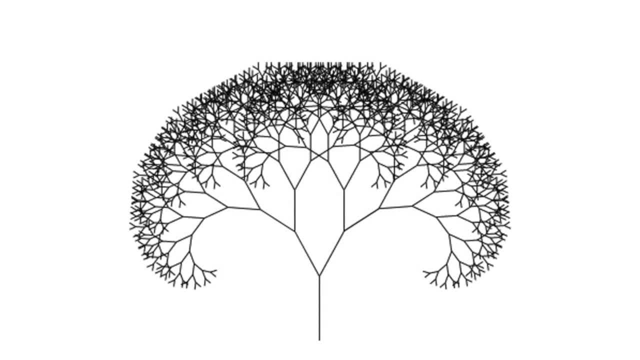 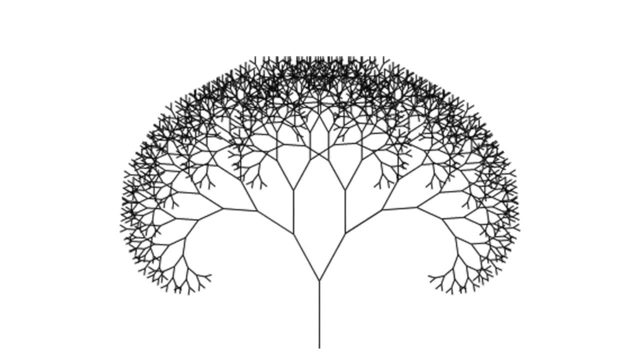 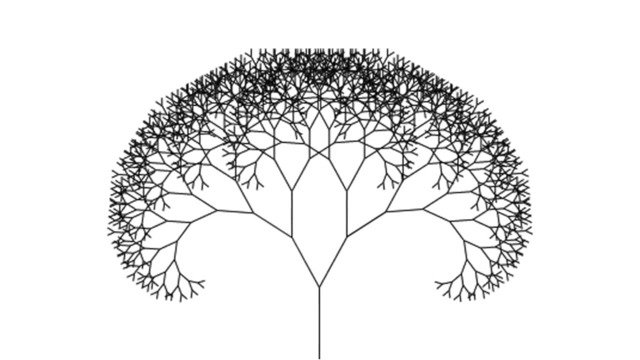 earth. The topological dimension is always a whole number, but the fractal dimension is different and measures, roughly speaking, how well a curve fills the plane or how well a surface fills space. There are many different forms of it, but one of the easiest to grasp is the box-packing. 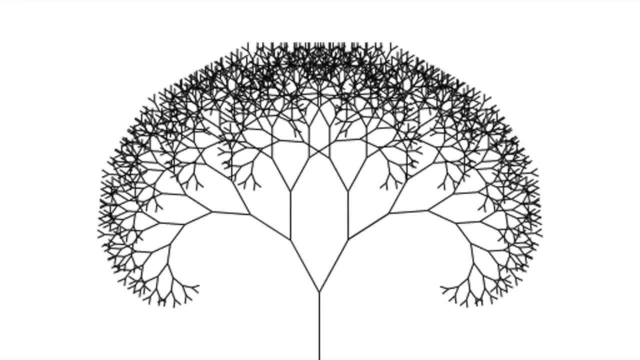 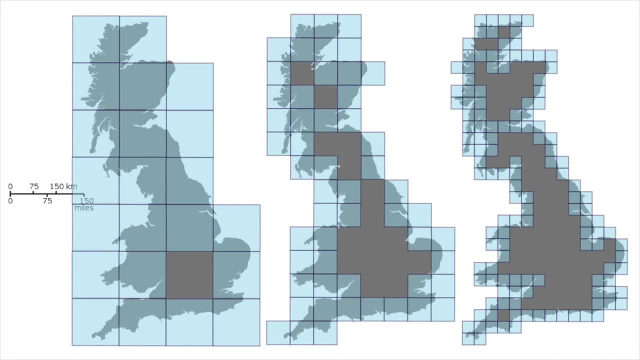 dimension, also known as the Minkowski dimension. To calculate it in the case of the coastline of Great Britain, we'd cover a map of the coastline with a grid of small squares and count the number of boxes that overlap the coast. Then we would halve the size of the boxes and count again If this was done with a straight line. 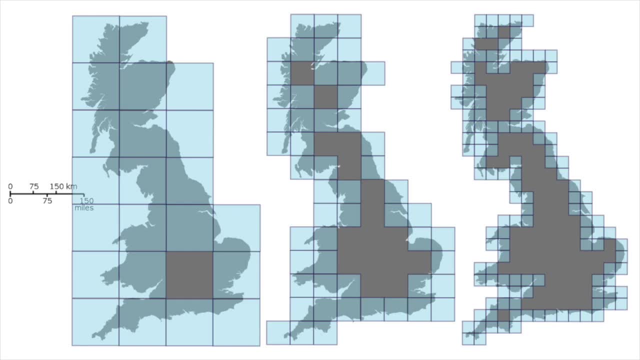 The number of boxes would simply double or go up by a factor of two to the one where the exponent one is the box-packing dimension. If it was done with a square, the number of boxes would quadruple or go up by a factor of two, squared, giving a dimension of two. 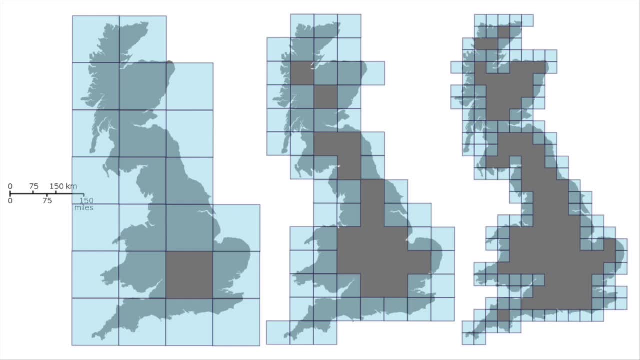 And in the case of a cube using a three dimensional grid grid, the number of boxes would increase by a factor of 8 or 2 cubed, because a cube is three-dimensional. The same thing could be done by dividing the size of boxes by 3 or any other.